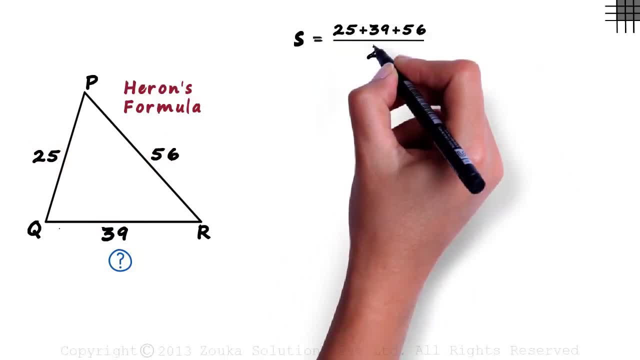 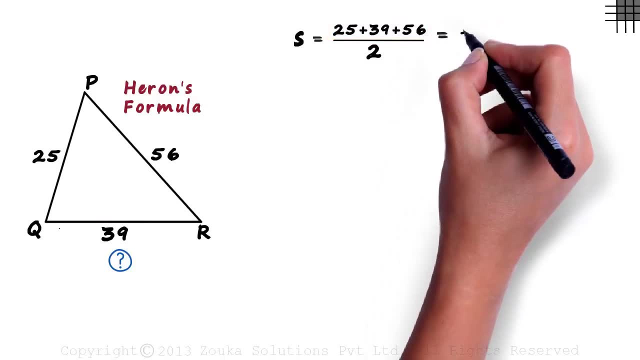 And the semi-parameter will be the parameter divided by 2.. This sum equals 120.. The semi-parameter will be 120 by 2, which equals 60 units. We have found the semi-parameter, But how do we use the Herron's formula? 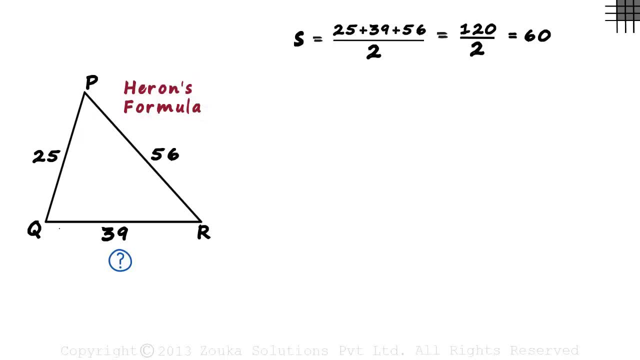 How do we find the area of triangle PQR? The area of triangle PQR will equal square root of S, multiplied by S minus A, multiplied by S minus B, multiplied by S minus C, Where A, B and C are the three sides of the triangle. 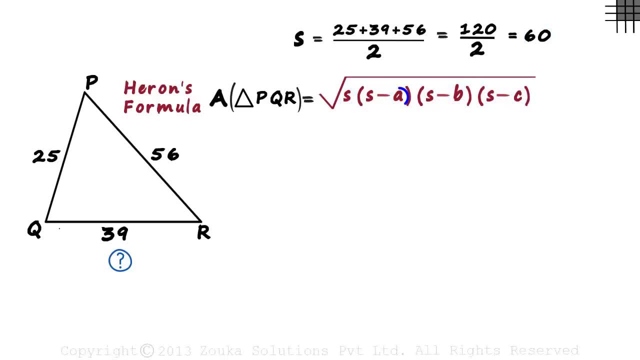 In this case S is 60.. A can be 25, B 39 and C 56 units. We just need to be a little careful with the calculations here, as the numbers when multiplied get really big. The area would equal square root of 60 multiplied by. 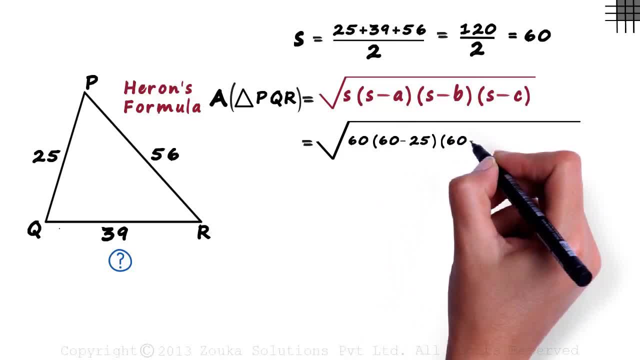 60 minus 25, multiplied by 60 minus 39, multiplied by 60 minus 56.. That will equal: square root of 60 multiplied by 60 minus 25 is 35. multiplied by 60 minus 39 is 21. multiplied by 60 minus 56 is 4.. 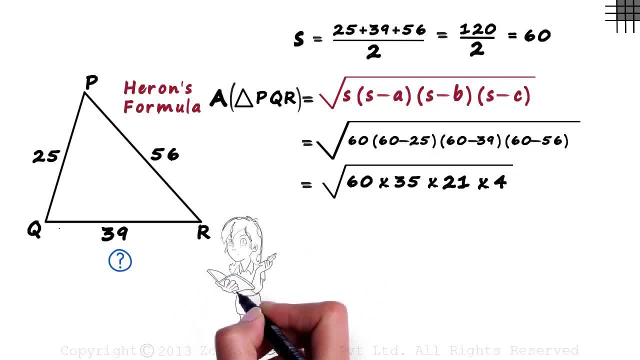 Think about the product of these numbers. It will be massive. The worst thing you could do here is multiply these numbers to find the product. In our videos based on square roots, we had seen that if the number is big we should use the prime factorization. 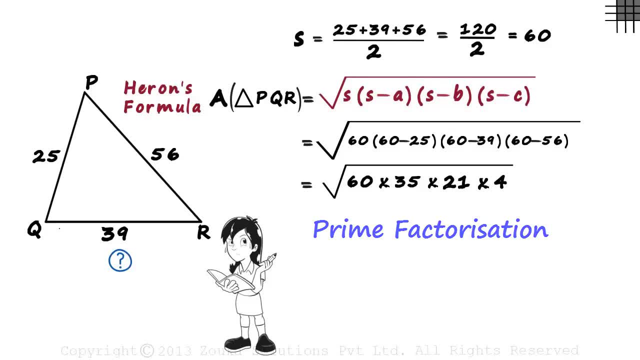 We have to use the prime factorization method to find the square root. And to use the prime factorization method, we have to reduce all the numbers to their prime factors. Let's look at the number 60 to start off. 60 can be written as 2 times 2 times 3 times 5.. 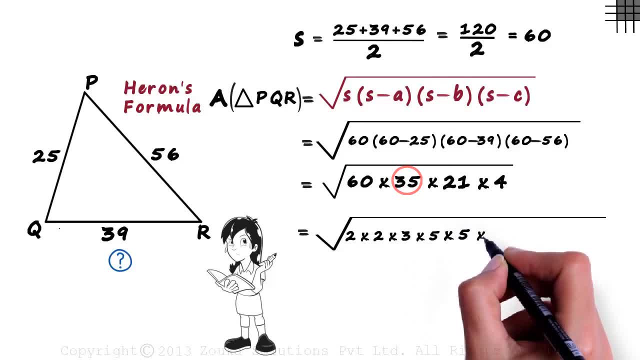 35 can be written as 5 multiplied by 7.. 21 can be written as 3 multiplied by 7.. And 4 can be written as 3 multiplied by 7.. And 4 can be written as 3 multiplied by 7.. 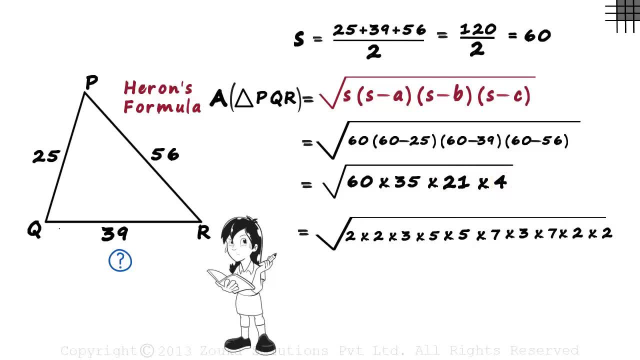 And 5 can be written as 2 times 2.. The next step in the prime factorization method was to start making groups of two same numbers. There are four 2s. They can be written as 2 multiplied by 2, multiplied by 2, multiplied by 2.. 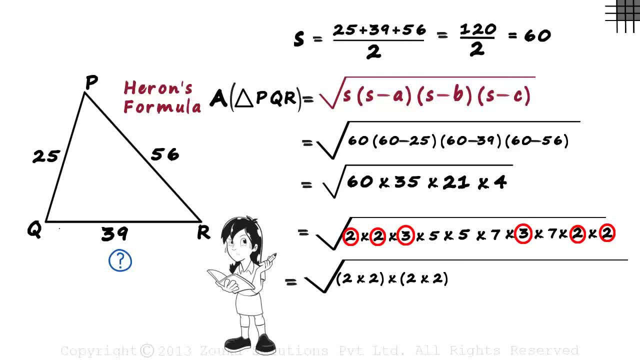 Apart from that, there are two 3s- We can write it as 3 times 3.. Two 5s written as 5 times 5. And two 7s as 7 times 7.. To get the square root of these numbers, 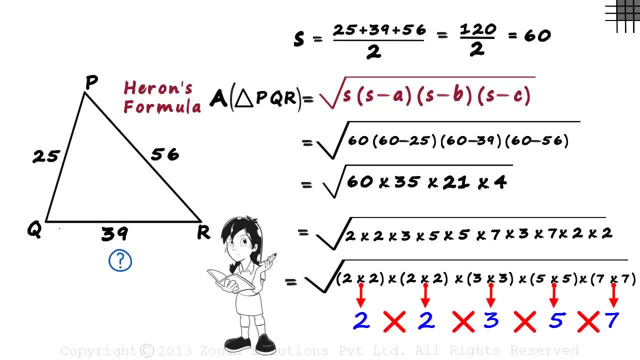 we pick one number from each pair, multiply them and remove the square root sign. It will equal 2 multiplied by 2, multiplied by 3, multiplied by 5, multiplied by 7.. That gives us 420 square units. The formula is pretty simple. 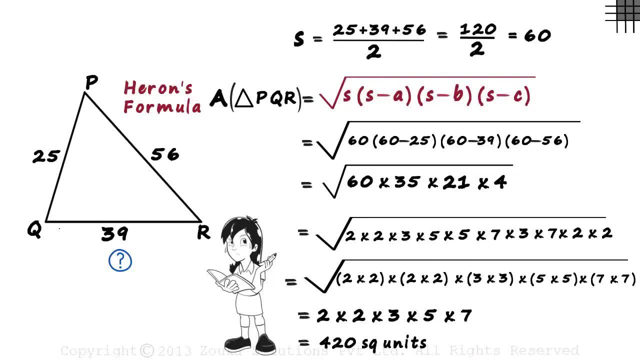 It is just the calculations we need to be careful about. Another important thing you need to remember here is the units of the answer. The units of area are always in squared terms. Think about the other formula of the area of the triangle. It's half base multiplied by height. 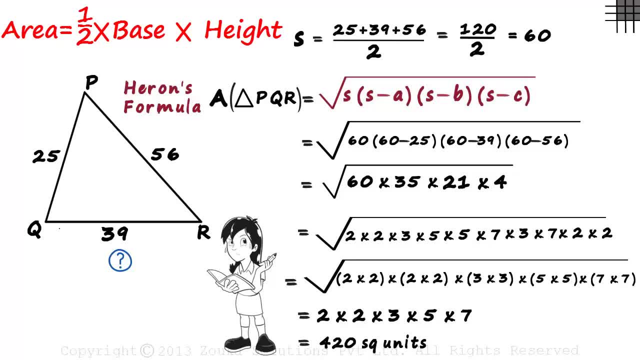 In this formula it's easy to understand the units, as units of base and height are multiplied to get squared units. But how do we get squared units here? Look at the formula carefully. Four lengths are multiplied, So the units would be square root of units raised to four. 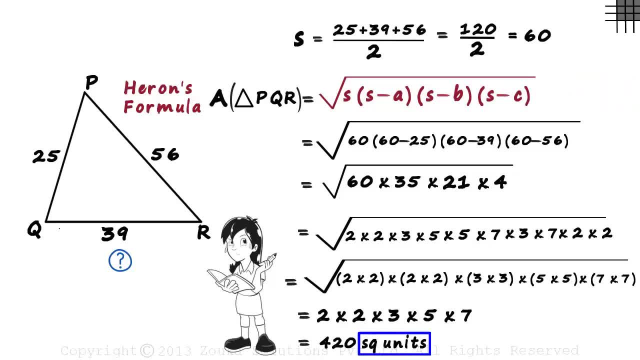 That gives us units squared, which is the same as squared units. 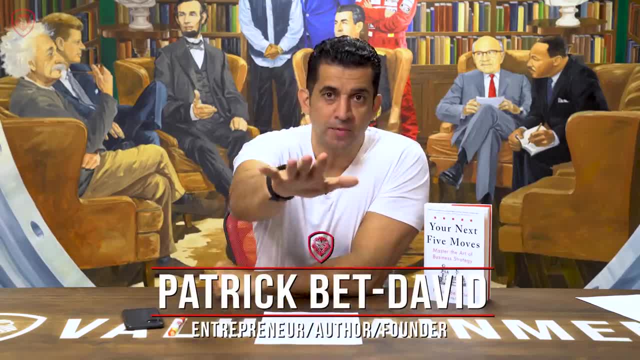 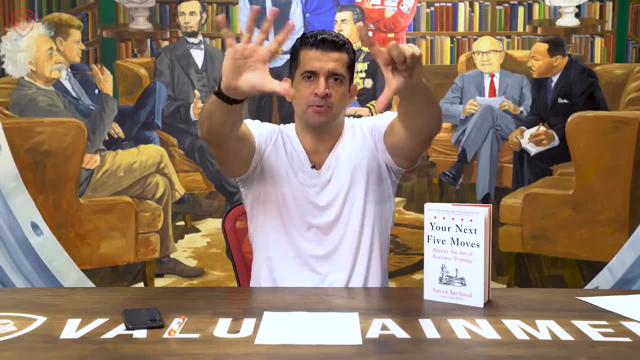 I'm gonna make a prediction: By the time you're done watching this video, you will not be looking at your co-workers the same way again, because at every single work environment and company, there are seven different types of employees and team members. I'm going to talk about that today. 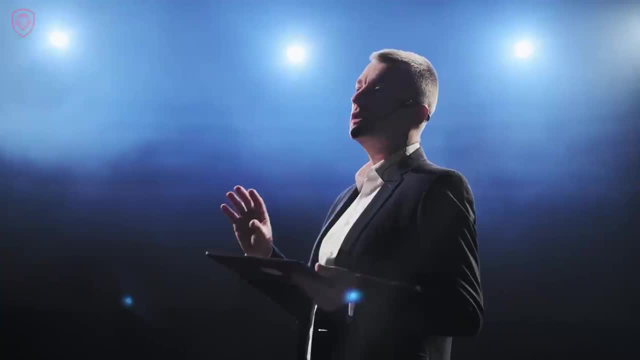 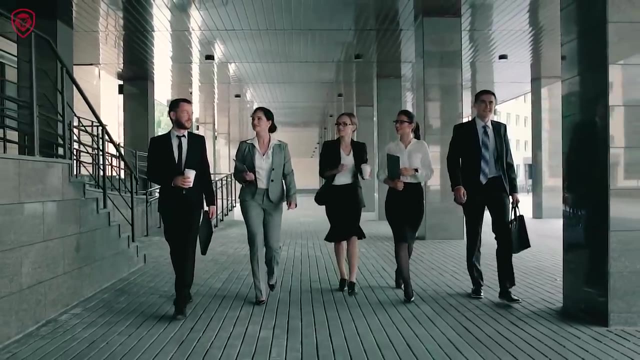 So this video is directed to two different types of people. One is the CEO and founder that wants to identify who he has on his team or who she has on her team. Two is for you to identify what kind of a team member you are at a company. So let's get right.